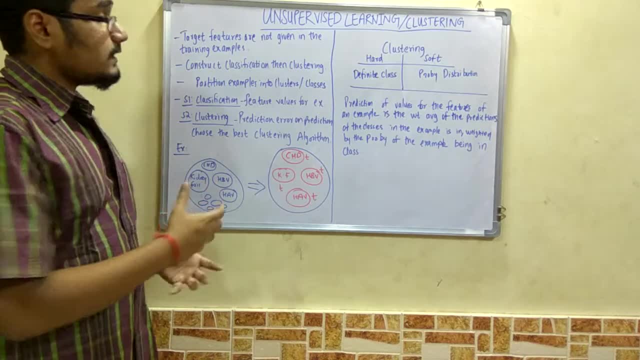 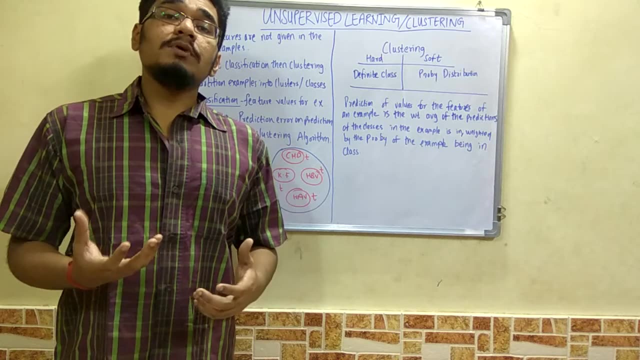 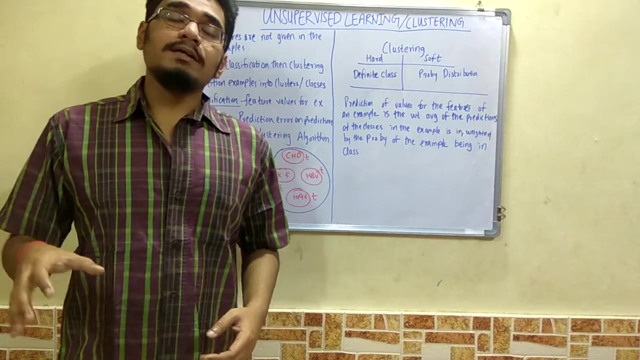 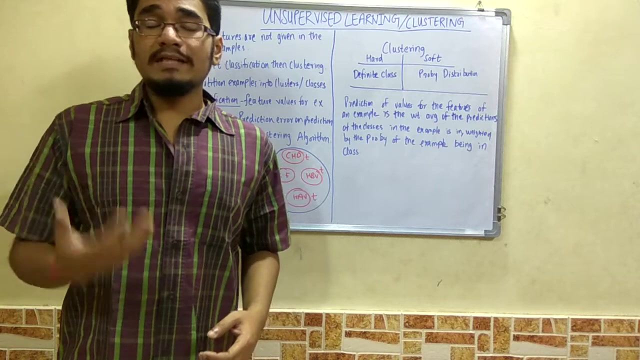 this we have to construct the classification and then clustering Means for unsupervised learning. since there is no supervision, first we have to do the classification of the examples which are there in the training set and, based on those training set examples, we will cluster them accordingly by using certain standard clustering algorithms, such as k-means or k-medoids algorithm or some other algorithm. 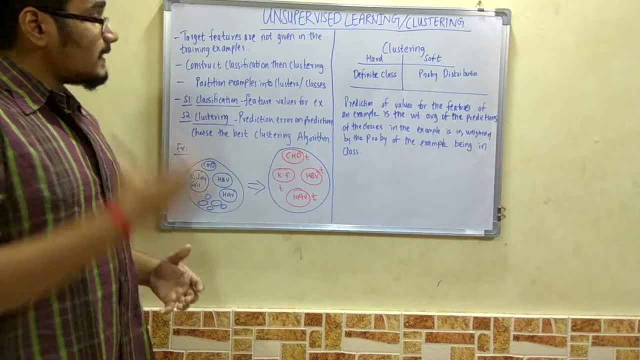 So the next step is partitioning of this samples into clusters or classes. means either you can classify it. if there is more requirement for the clustering, then clustering can be done. Now, clustering is basically done to predict the error on this examples. So we will see that. so first, in this unsupervised learning, we have to do the classification. that is the specification that we will use to predict the error. Oliver. 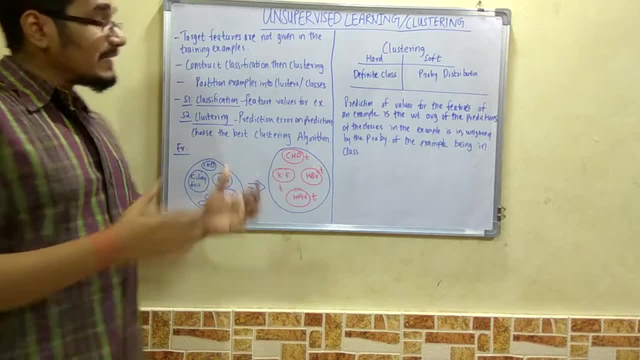 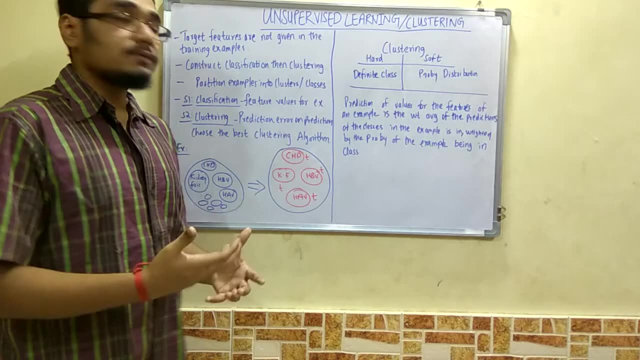 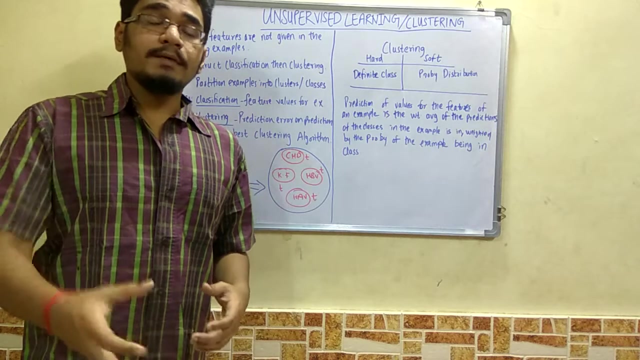 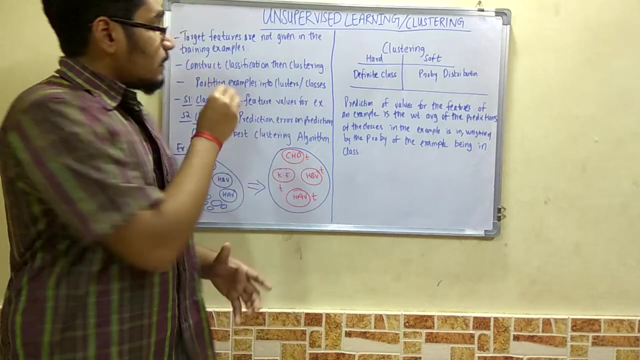 step 1 is to classify the examples which are there in the training set. so what this classification gives is it gives the feature values for the training set examples. now, feature values are those values which are inherited or exhibited by those examples from the training set. now, this feature values are unique for 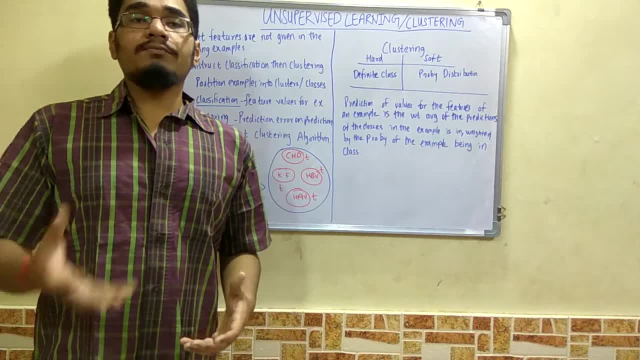 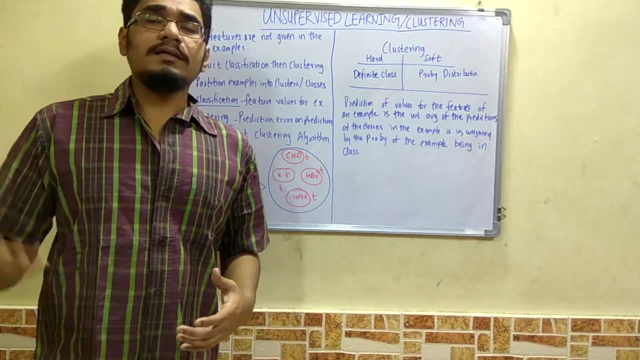 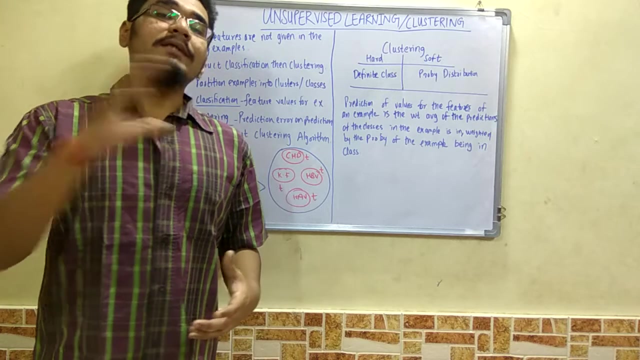 different examples now, for example, consider training set of disease. now the disease can be categorized into or there are many types of disease, like lung disease or heart disease or brain disease or some other cancer. so this all disease have a peculiar property that will exhibit. so this properties are: 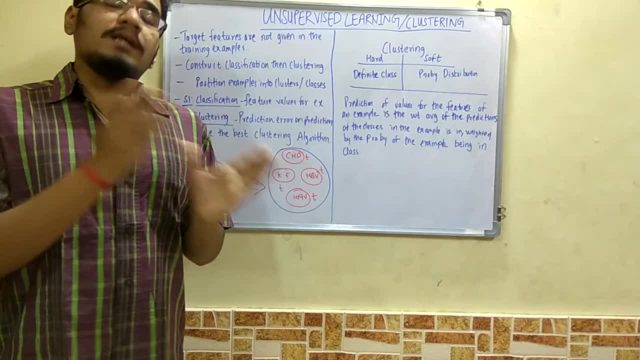 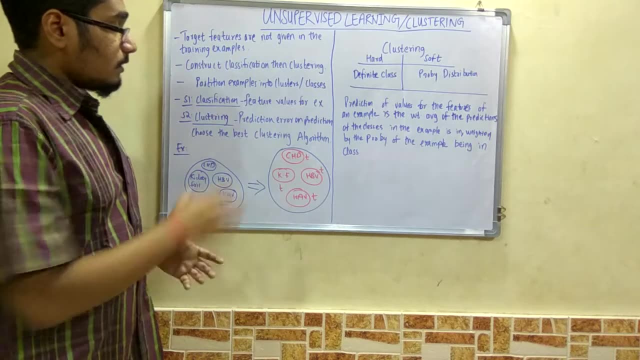 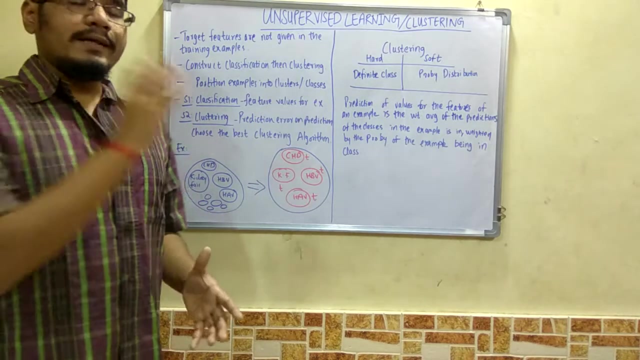 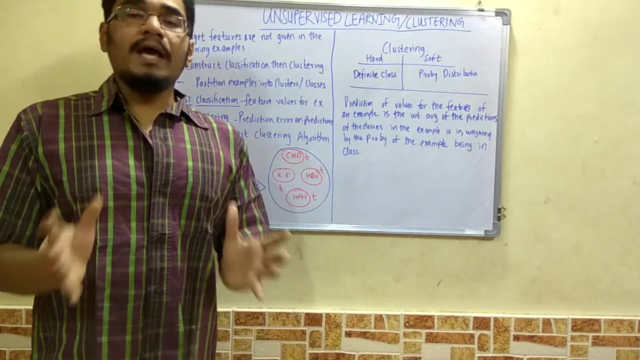 called as the feature values. so we will classify them and then we will cluster them. second step is clustering. that is, predication of the error on prediction. now we will choose the best clustering algorithm. now in clustering we will predicate the error means, for example, in we have our training set. in the training set we will 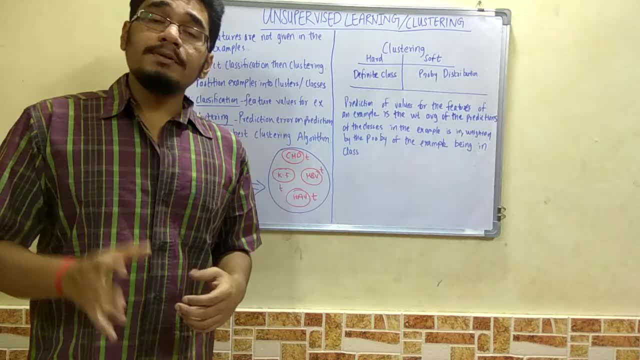 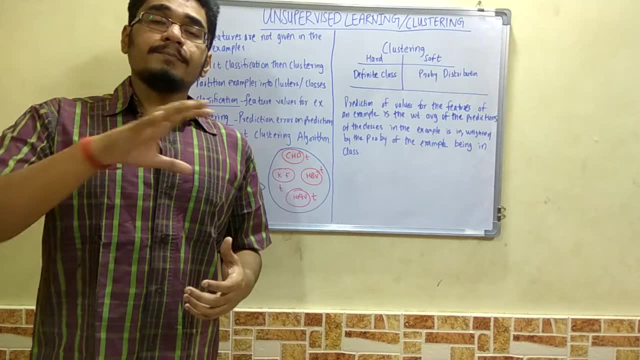 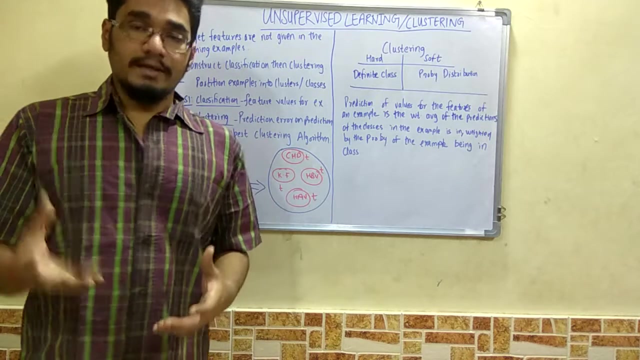 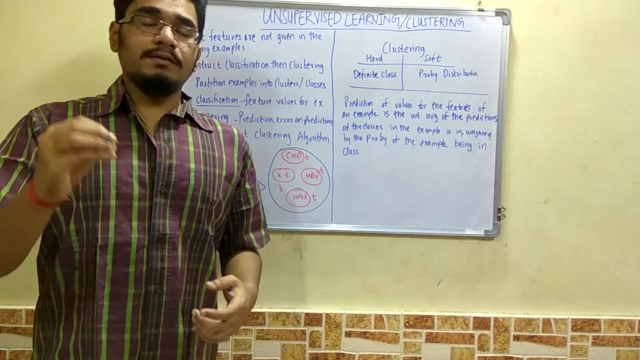 first classify those examples. now these examples are further than the clustering. now clustering is done mainly for opening of the errors which are there present in this examples. now this errors are basically probably distributed, like it is based on the prediction means for some random variable x. if we generate the output, then it may not be the. 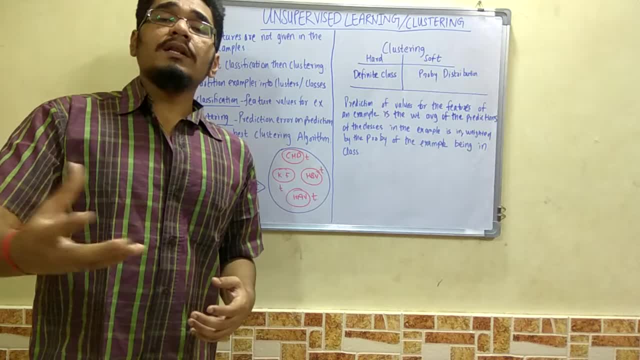 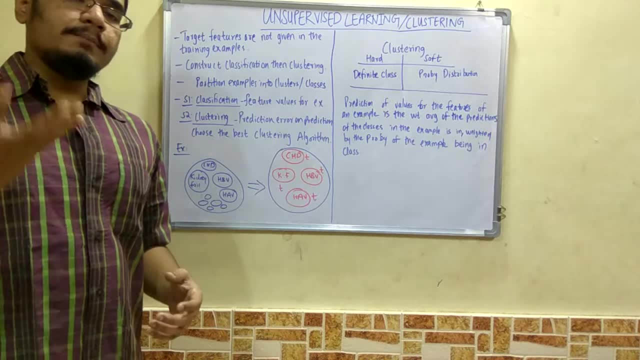 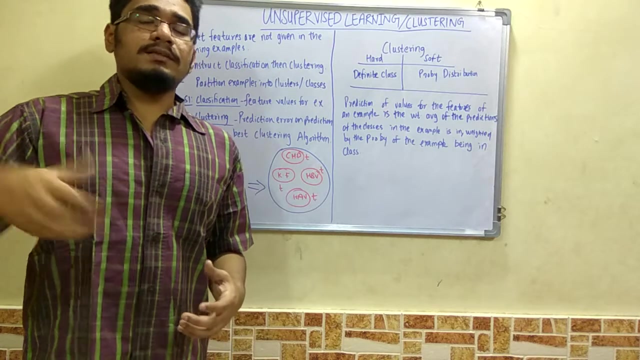 expected one as of the desired user. so we will then discard those output and we will generate the new one. so that is basically the prediction. error means we will predict. there is no such particular fixed or algorithm for this clustering. it is generated dynamically if we find the previous one was worse than the new one. 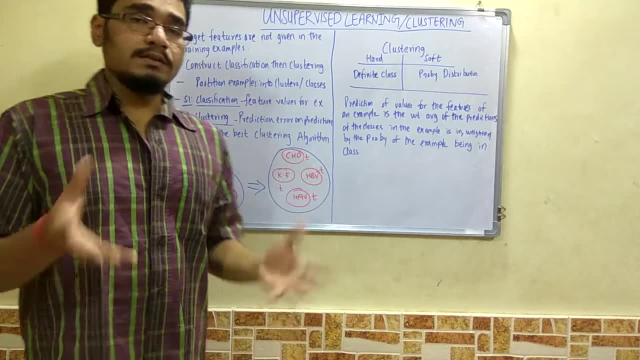 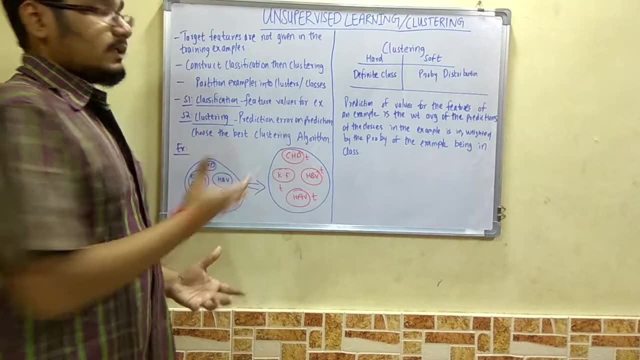 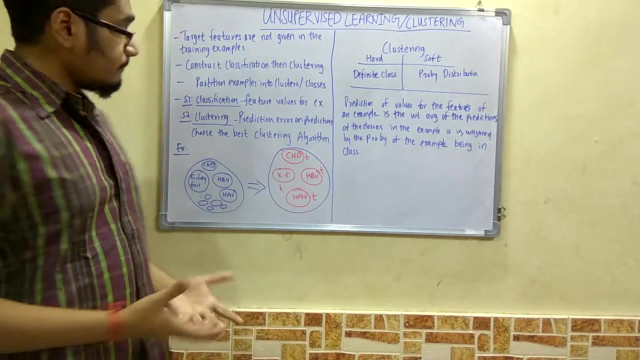 then we will consider the new one, and so vice versa. the thing happens now: out of this: we choose the best clustering algorithm which is done for the clustering, that is, k-means, k-metoids or birch or some other techniques which are available in data mining and machine learning now. so there, 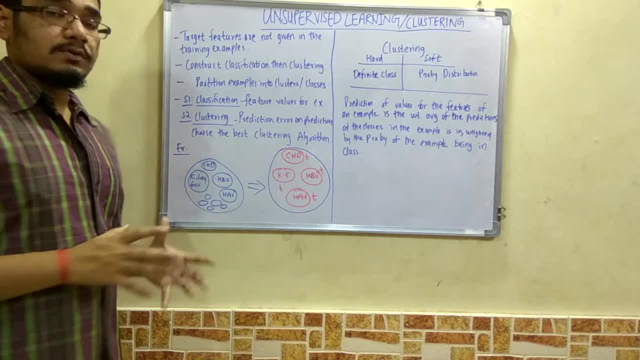 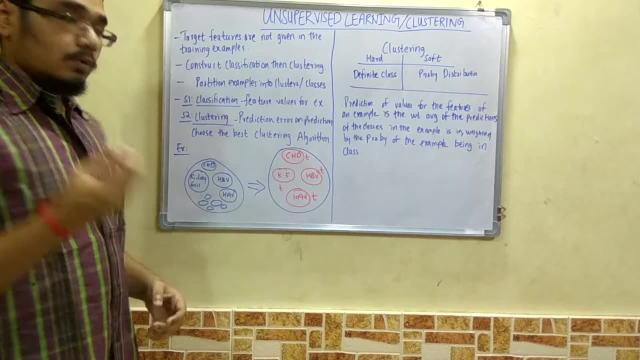 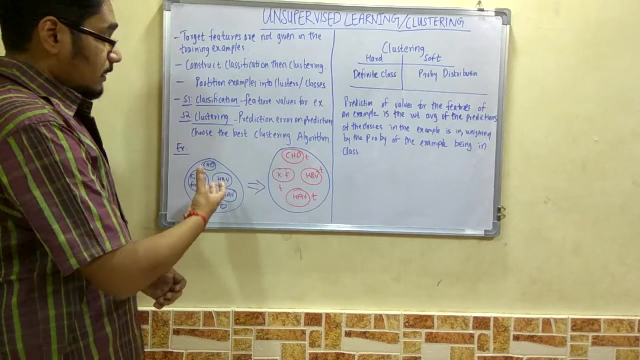 is an example. this example consists of a analyst, that is, a disease analyst. is there diagnostic? basically? so in this, first we will categorize the diseases which are there, that is, it is coronary heart disease or hepatitis b virus, or hepatitis a virus, or if it is a renal or 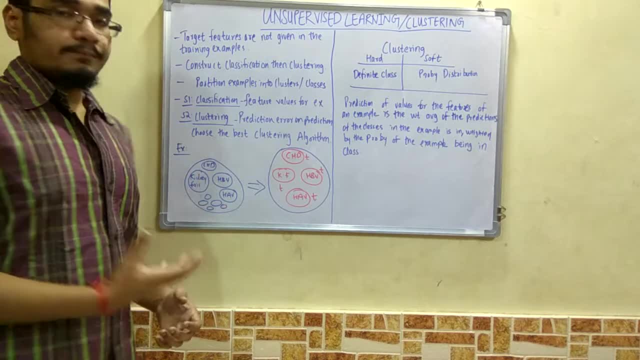 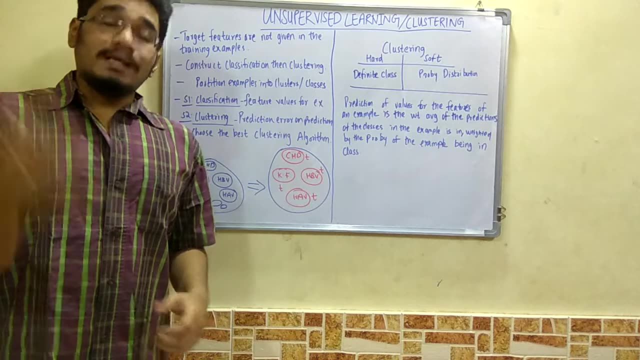 aşkrier virus or hepatitis b virus, or if it is a renal or 학er virus or hepatitis b virus or failure, or if there are some other diseases. so first the analyst or the agent, the robotic agent, first needs to classify those diseases accordingly and 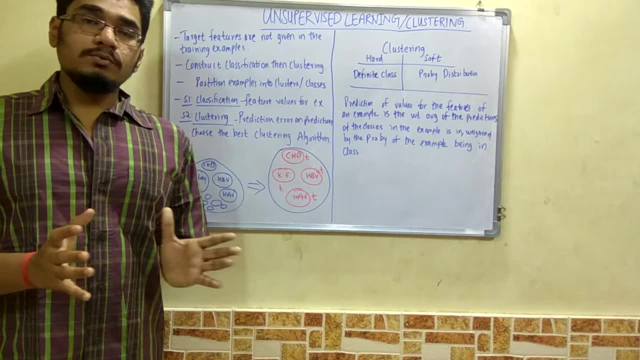 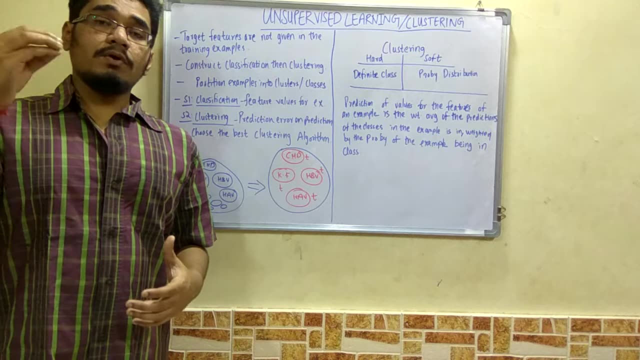 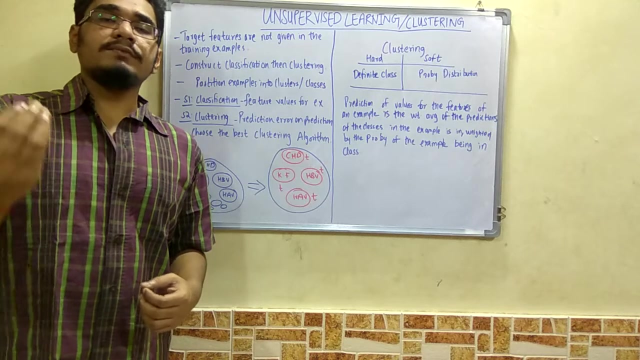 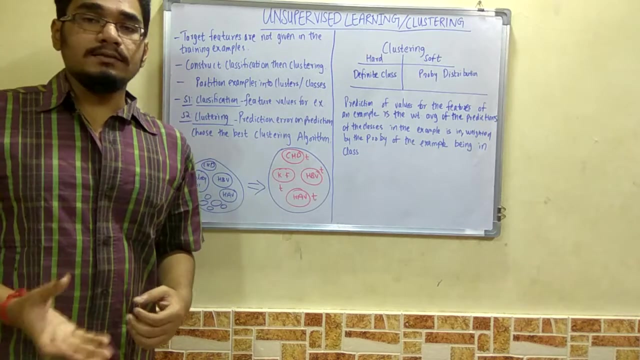 these diseases are then fed into a training set. now this helps the agent to classify means for what disease, what particular output should be there or what kind of special treatment should be given for each of these diseases. obviously we cannot give the medicine which is fed to kidney failure to heart. 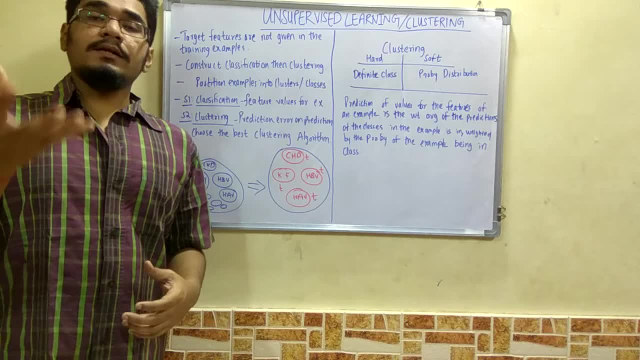 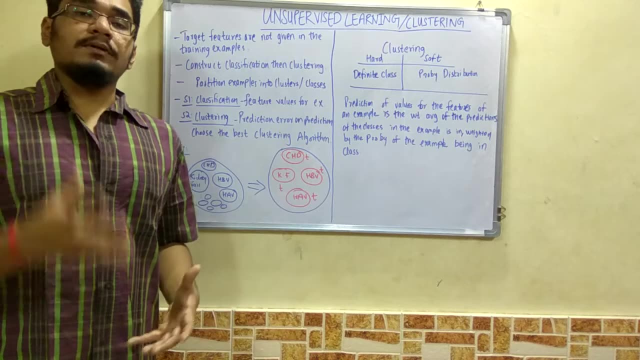 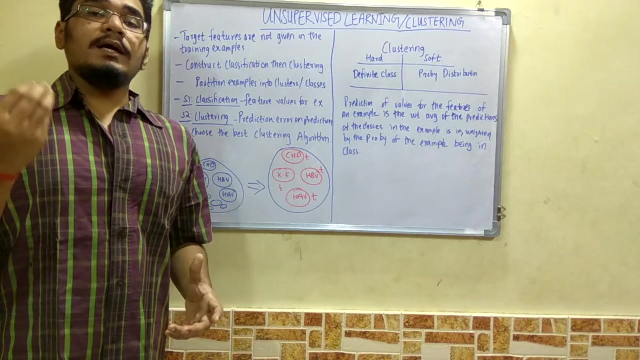 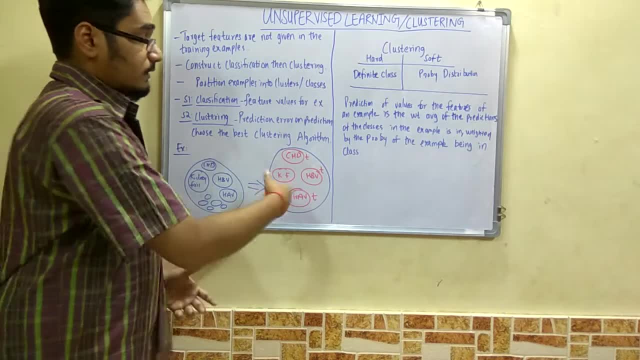 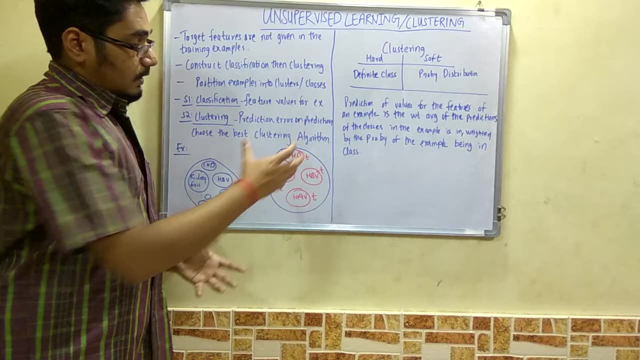 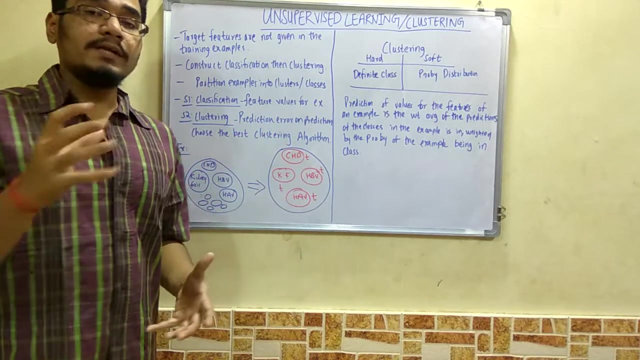 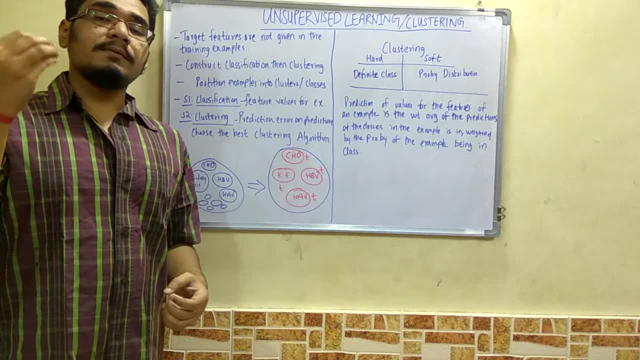 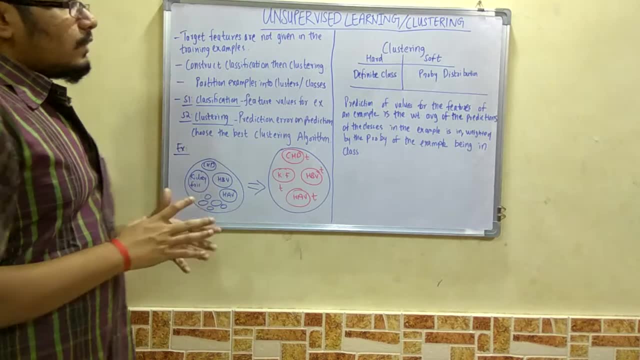 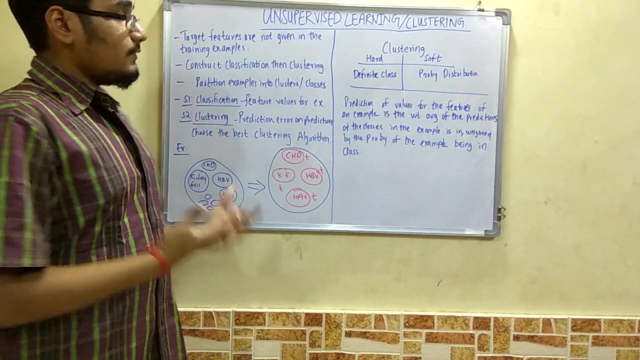 treatments and for individually allocating the precautions as well as the suggestions which needs to be cared for each of these diseases. now, moving further, we will see what are the two types of clustering. so in mining, that is, the artificial intelligence, we have two types of clustering. that is the hard. 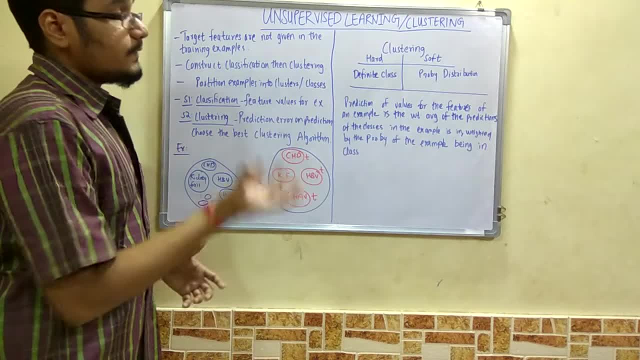 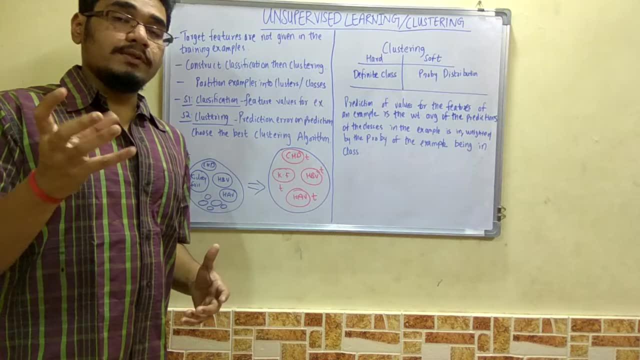 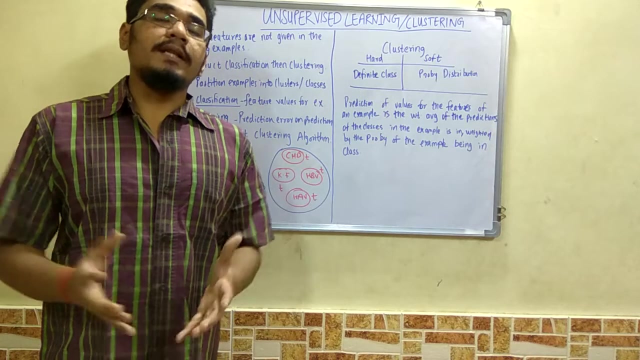 clustering as well as the soft clustering. now what is the difference between these two? now, in a hard clustering, we have a definite class consisting of the training set. examples means we have the examples and variables from the training set will assign it to a definite class. now that class is a. 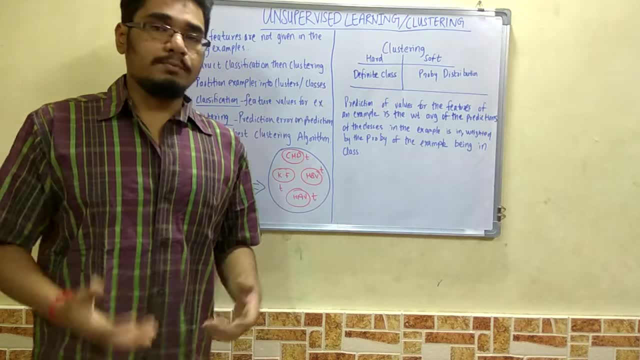 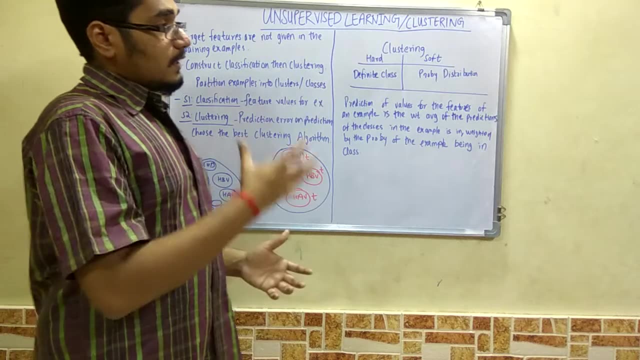 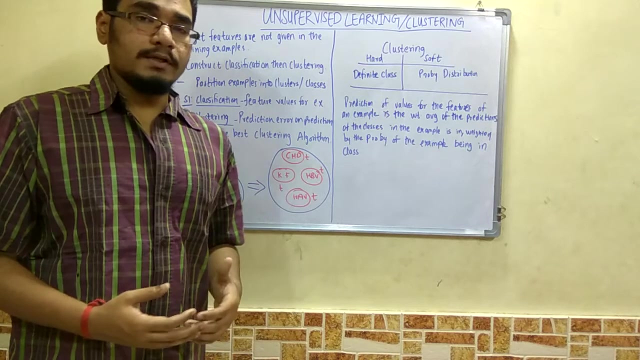 class it belongs will be permanent throughout the execution and throughout the process. there will be no change in that. and the another one is the soft clustering. soft clustering basically differs from hard clustering by the probability distribution of the examples from the training set, means based upon the probability it will change. keep on it will. 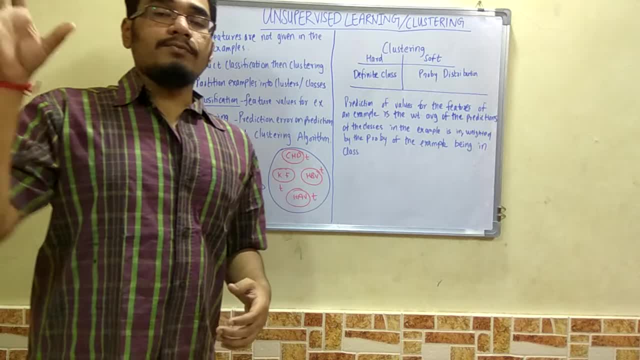 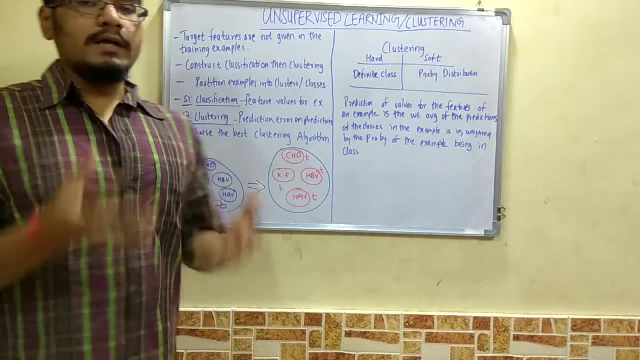 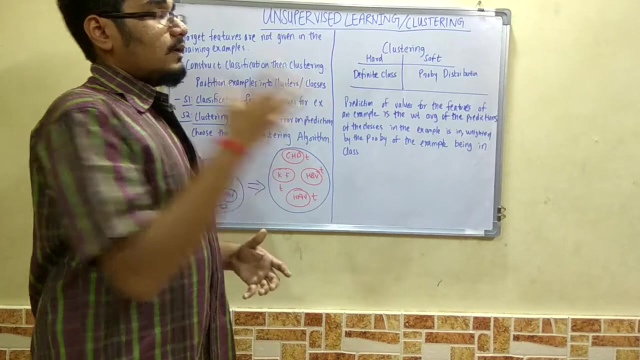 keep on changing on this. training set means from this disease to this disease means it's not compulsory that a person having a heart disease will not have a kidney failure, so it may be building on the dependency what the patient has means if he has a single disease or multiple. 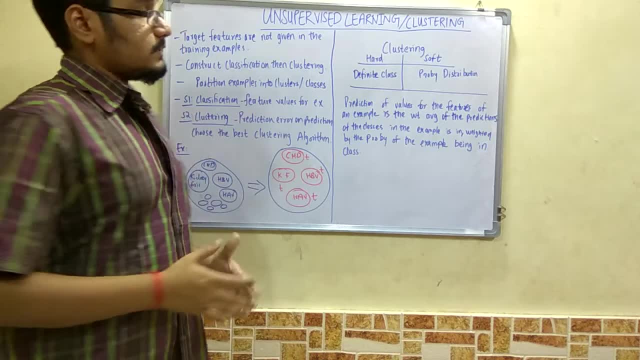 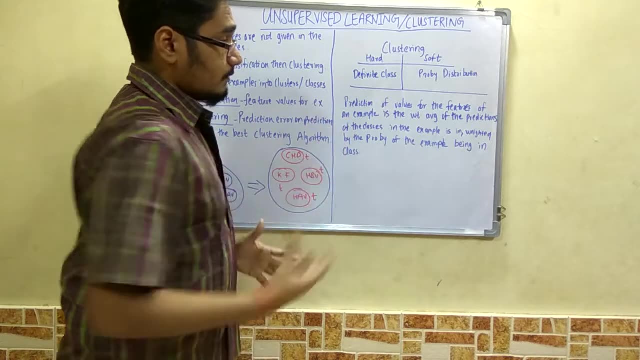 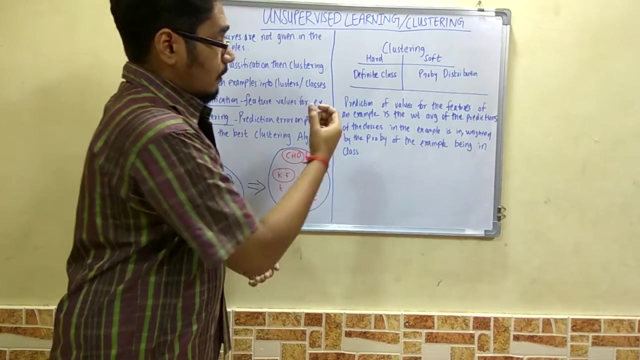 disease and that will be considered under the soft clustering. next, there is a broad statement made in unsupervised learning. so it says that the prediction of values for the features of an example is the weighted average of the predictions of the classes in the example is in, weighted by the probability of the 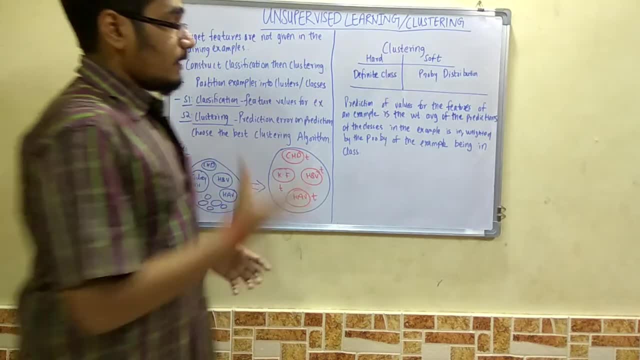 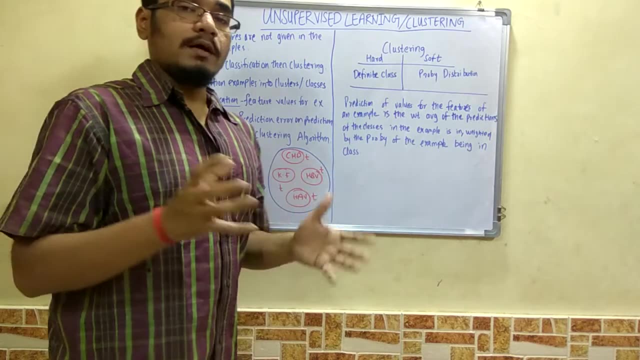 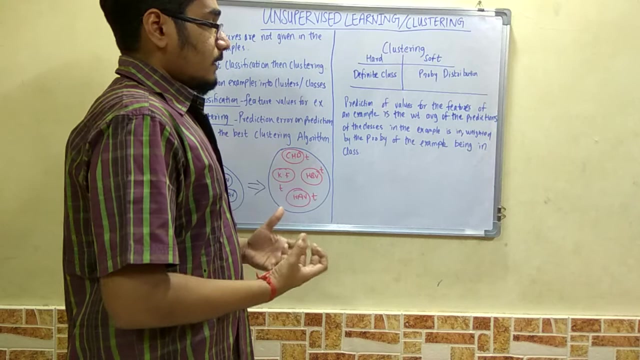 example, being in the class. now what does it mean? see the prediction of values for the features of an example means we have a training set in that will predict the values of this training set variables. now these individual features is the weighted average of the class, and the weighted average of the class is the.